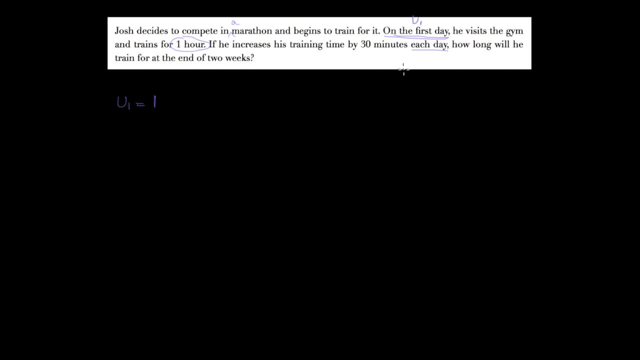 It's not how many he goes every other day. It says 30 minutes each day. So that implies that he's going every day. Okay, and if he increases his training time by 30 minutes each day, that's a constant increase. 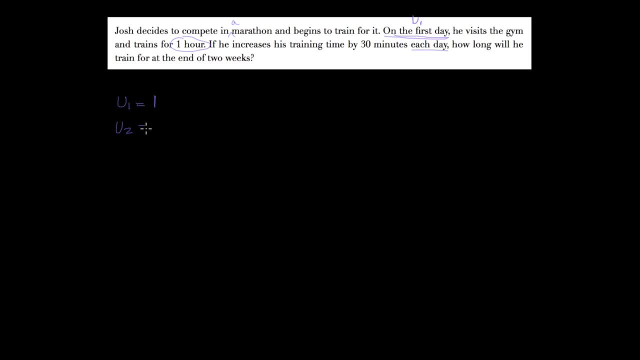 The first day, so the second day would be one plus now 30 minutes. I can't just write 30, I have to be very careful here. This one is in terms of hours and 30 is in terms of minutes. 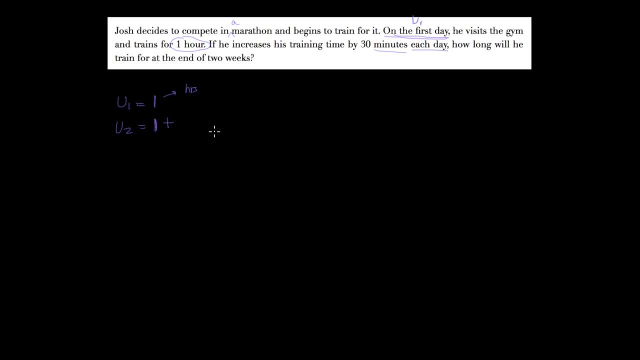 So I have to convert both of them to a similar value. So hours gives me a whole number, so I'm going to go with that. 30 minutes is half of an hour, so it's going to be 0.5.. So that's how much he would train on the second day. 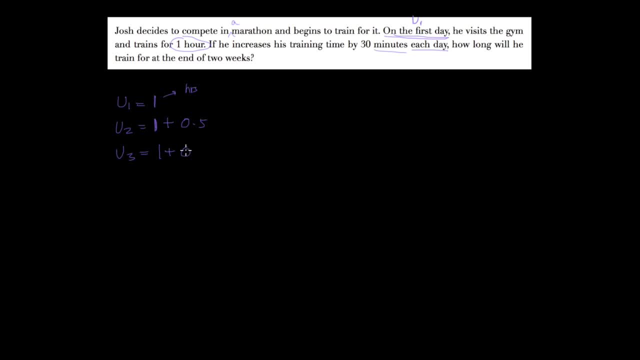 The third day he would train for this same value and increase it by half an hour again. So this increase is constant. so it is an arithmetic series. Okay, so we have this information and it says how long would he train for at the end of two weeks. 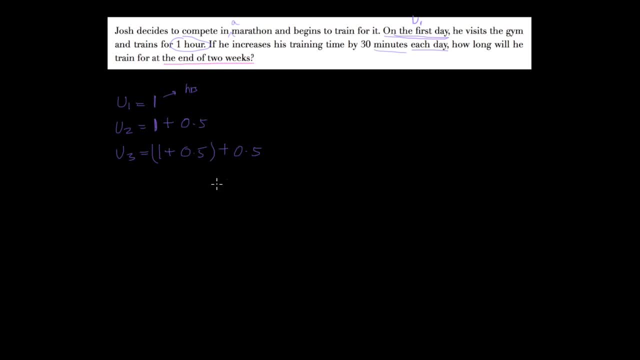 At the end of two weeks. So two weeks is 14 days. So it's asking me, on the 14th day, how long is he going to train for? So what I'm trying to find is u sub 14.. Now let's go back and refresh our memory about the formula. 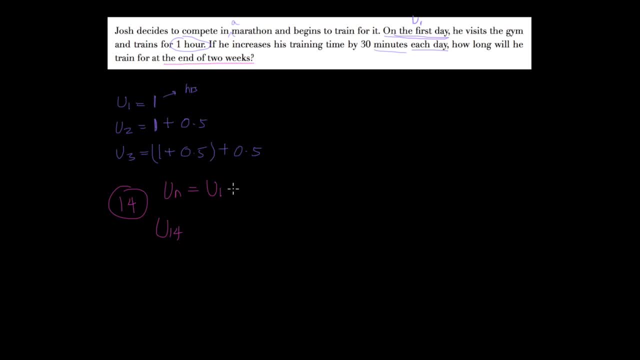 It's u sub n equals u sub 1, plus n minus 1 times d. So I have u sub 14 equals u sub 1, but u sub 1, Thursday, one hour, so 1.. Plus my common difference d is going to be 0.5, because that's what he increases his gym time by each day. 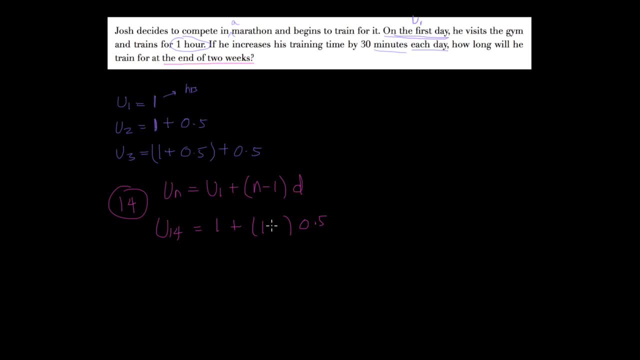 And my n is 14, so 14 minus 1 is going to give me 13.. So u sub 14 equals 1 plus half of 13 is 6.5.. So u sub 14 is 7.5 hours. 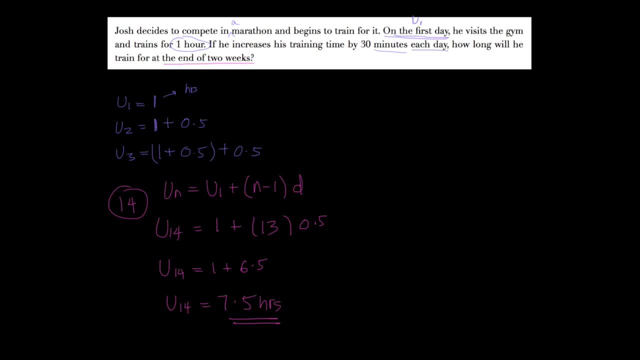 So this means that on the 14th day after Josh starts his training, he's going to train for 7.5 hours. Wow, that's a lot, Okay. so this is how you deal with word problems. Hopefully that helped. Thank you and see you in the next video.